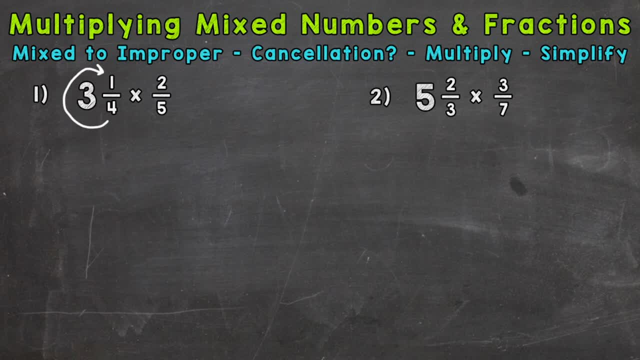 starting at the bottom and working our way up. So we multiply and then add. So 4 times 3 is 12 plus 1 is 13.. We keep our denominator of 4 the same, So 13 4ths is equivalent to 3 and 1 4th. We didn't change the value of the problem at all. 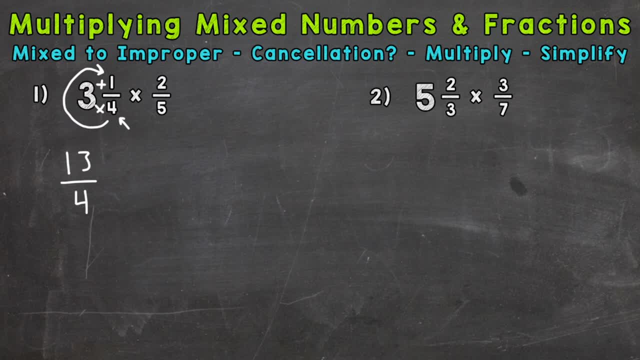 We just changed to an improper fraction. Now we can bring 2 5ths down and we have a multiplying fractions problem here. So we can multiply straight across. But before multiplying straight across, you can always check to see if you can use cancellation. You can think of this as simplifying. 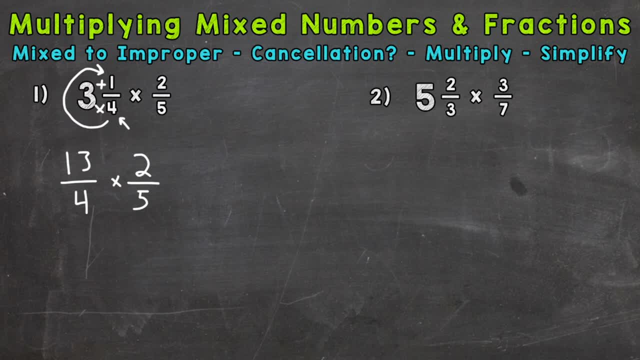 the problem before you multiply. It helps us get easier numbers to solve So we're going to work with and also cuts down on any simplifying at the end of the problem. So, generally speaking, it makes the problem simpler to work through And in the case of number 1, we can use cancellation. 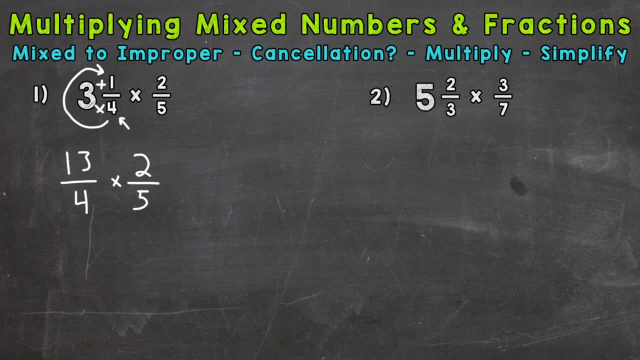 So you need to look for common factors between the numerators and denominators. So 4 and 2 have a common factor of 2. A greatest common factor of 2.. So let's divide 4 and 2 by 2.. 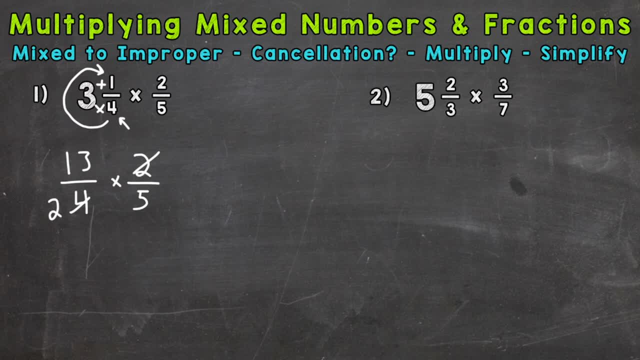 4 divided by 2 is 2.. 2 divided by 2 is 1.. So let me rewrite the problem. We have 13 over 2 times 1 over 5.. 13 and 5 do not share any common factors other than 1.. So we cannot use. 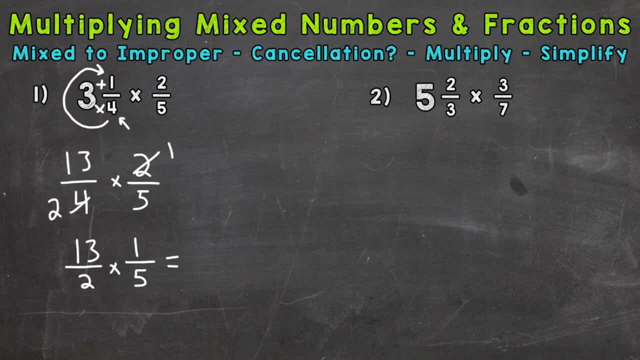 cross cancellation with the 13 and the 5.. So now we can multiply straight across: 13 times 1 is 13.. 2 times 5 is 10.. So we end up with an improper fraction here. So let's change this back to. 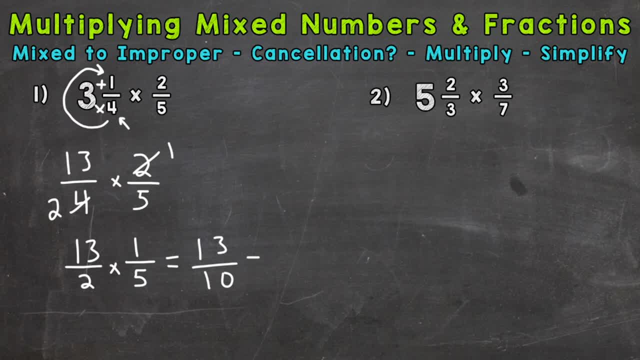 a mixed number for our final answer. So we do that by doing the numerator 13 divided by 10.. So how many whole groups of 10 out of 13?? Well, 1. And we have a remainder of 3.. So that's the numerator of our fractional part, And we keep the denominator And we 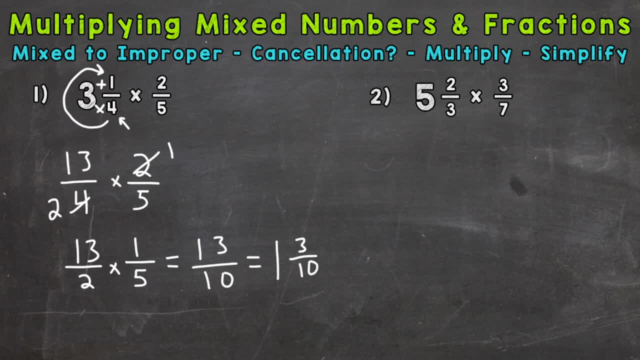 keep the denominator of 10 the same. Always check to see if you can simplify the fractional part of a mixed number. But in the case of number 1, 3 tenths is simplified, So our final answer is 1 and 3 tenths. I do want to show you. before we move to number 2, let me rewrite: 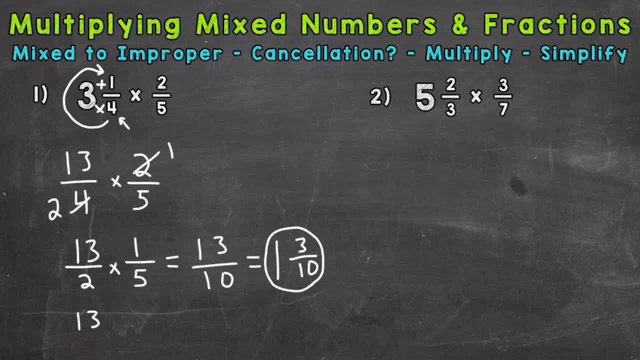 the problem below here. So we have 13 over 4 times 2 over 5.. So we have 13 over 4 times 3.. So if you do not use cross cancellation, that's fine, You'll get to the same answer. 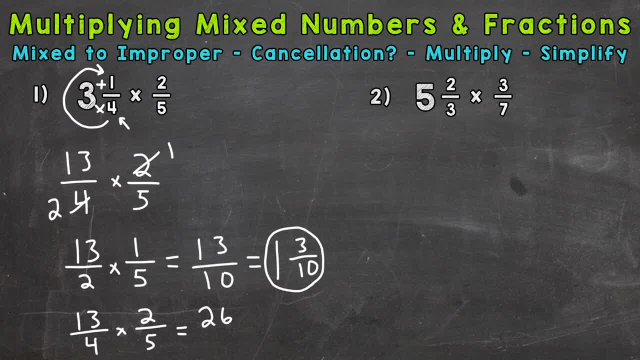 So 13 times 2 is 26.. 4 times 5 is 20.. And then we would do: 26 divided by 20, row of 20 contends twenty out of 100 to get to a mixed number. So how many whole groups of 20 out? 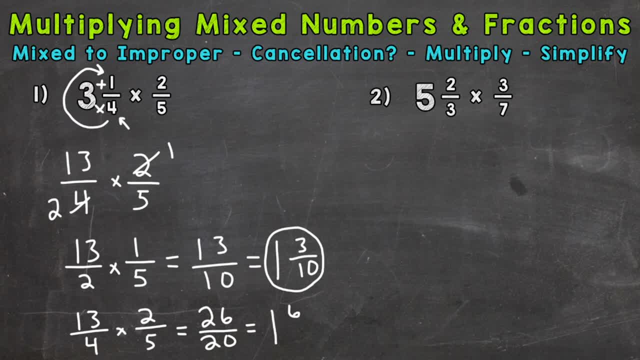 of 20, 6? 1.. With the remainder of 6, keep the denominator of 20 the same. Now we can simplify the fractional part after, If we do not use cross-cancellation, we can get to the same answer. so we mushrooms out the axial extension here for the whole group. You can keep the denominator of 18 because it altevates all the times, and then we just simply keep it the same. So that's the basic idea of the amazed question: the 12 minutes played by each So you can execute as lucy, which means if you do the 20 second apiece. 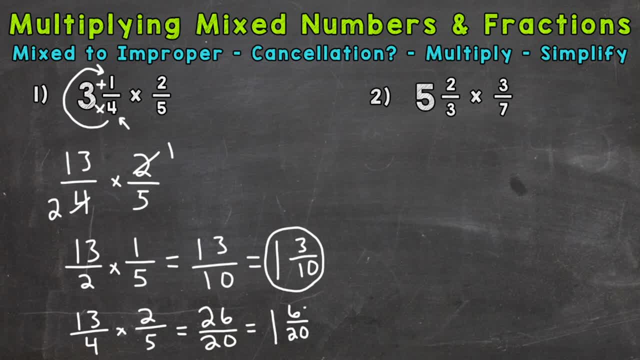 we have a greatest common factor of 2 between 6 and 20, so divide each by 2 and we end up with 1 and 3 tenths. so same answer, just we had to simplify at the end there instead of using cancellation and simplifying the problem before we. 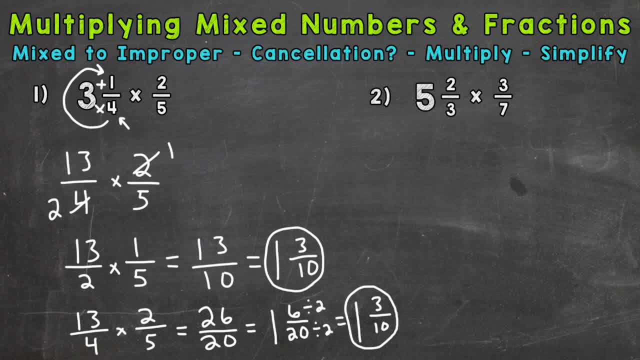 multiplied. so on to number 2, where we have 5 and 2 thirds times 3 sevenths. so again, first thing we need to do, change any mixed numbers to improper fractions. so we'll start at the bottom, work our way up, multiply and add. so 3 times 5 is 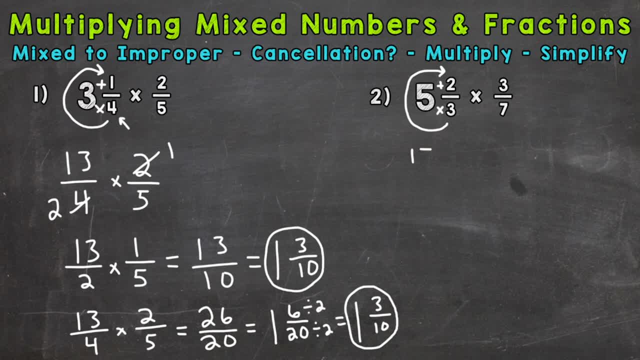 15 plus 2 is 17. keep the denominator of 3 the same times 3, sevenths. now we can look to see if we can use any cross cancellation here. and 17 and 7: greatest common factor is 1, so we cannot use any there, but we have a 3. 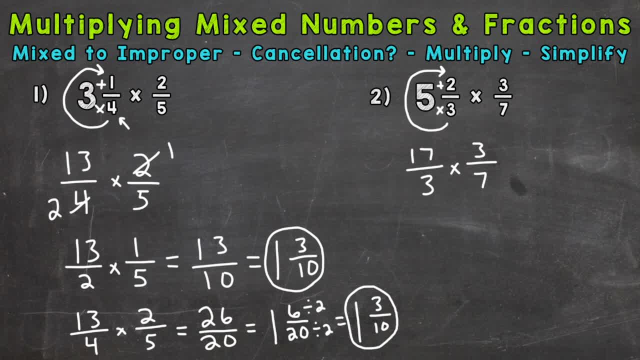 and a 3, so greatest common factor is 3. we can divide each by 3, so 3 divided by 3 is 1, and 3 divided by 3 is 1. so we have this problem here and we can multiply straight across: 17 times 1 is 17 and 1 times 7 is 7. so we end up with: 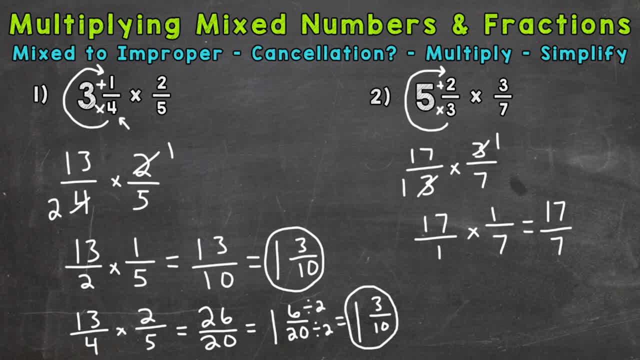 an improper fraction which we want to change back to a mixed number. so we need up with an improper fraction which we want to change back to a mixed number. so we the numerators 17 divided by 7, how many whole groups of 7 out of 17? 2 that gets us to 14. 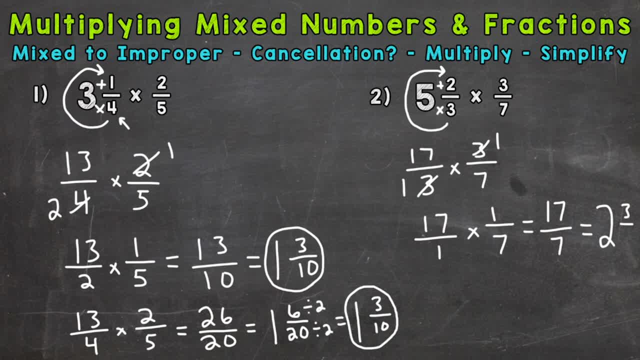 so we have a remainder of 3 and keep the denominator of 7 the same. always look to see if you can simplify the fractional part of a mixed number any further, but 3 self's and the whole thing. so let's start telling now what's our. 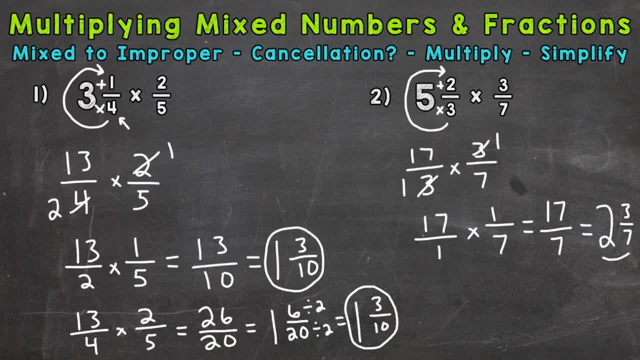 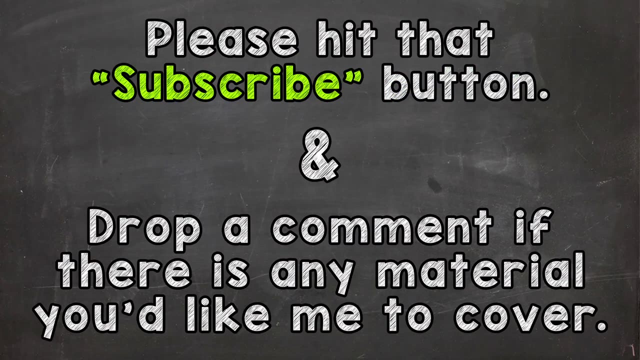 is in simplest form. So we are done here. The answer is two and three sevenths. So there you have it. There's how you multiply mixed numbers and fractions. I hope that helped. Thanks so much for watching. Until next time, peace. 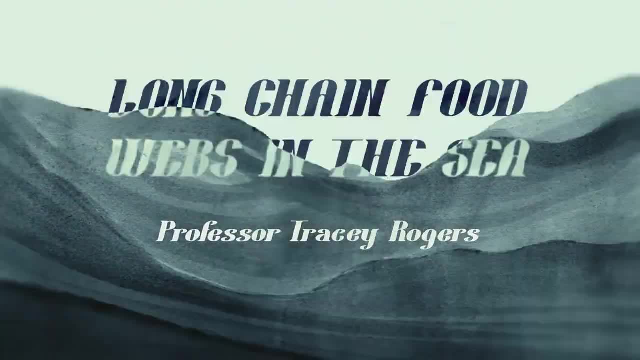 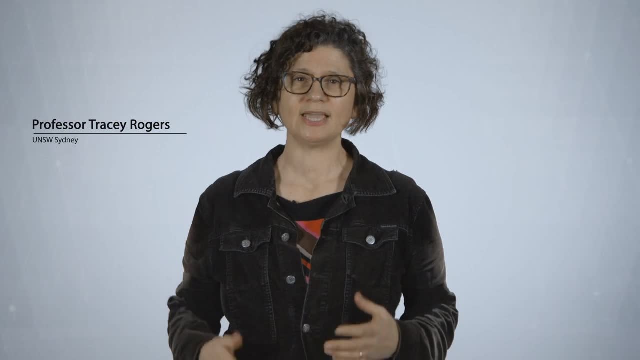 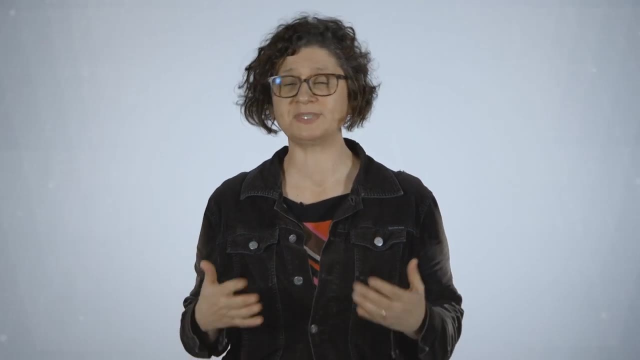 Do you eat tuna, fish and chips or shark fin soup? Any idea how much material it took to produce your 100 gram tin of tuna? Well, because marine food webs and hours on land are very different, you might be surprised. In the ocean there are more trophic levels. 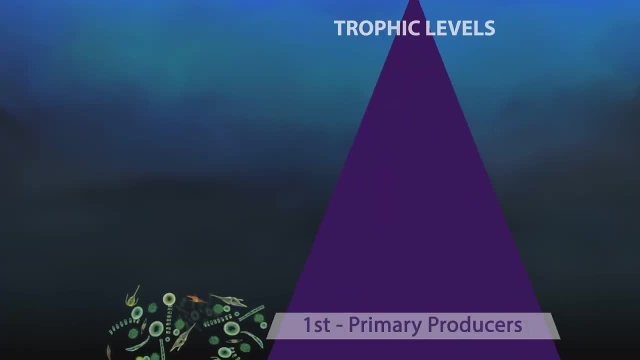 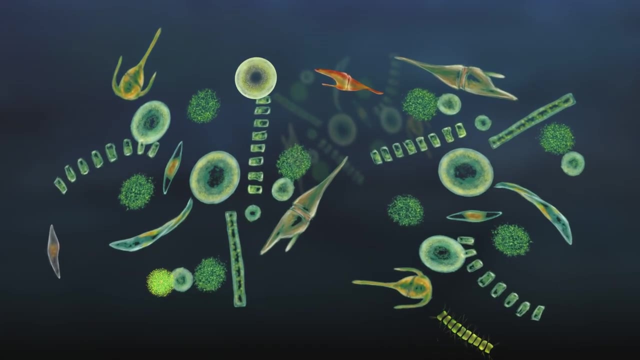 more steps in the food chain than hours on land. It's because at the base of the marine food chain, the phytoplankton are really tiny. Phytoplankton are the foundation of the marine food web, just like grass, leaves, nuts and fruits are for us on land. But because